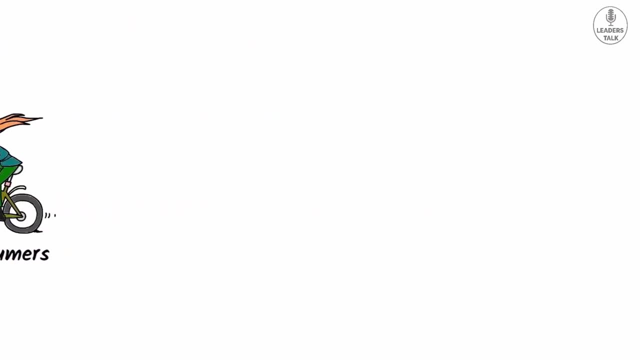 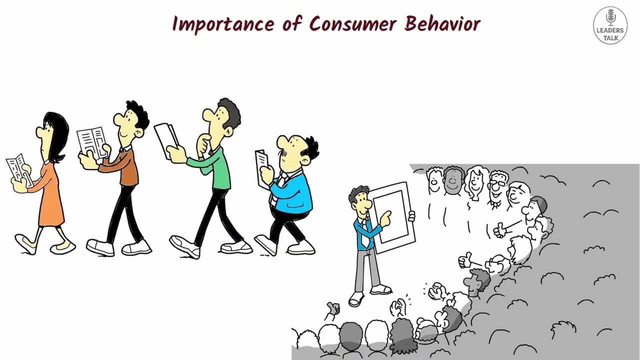 product or service, regardless of whether they made the purchase themselves. For example, a parent buying a toy for their child is the customer, while the child is the consumer. Importance of Consumer Behavior: Understanding consumer behavior is crucial for businesses and marketers. Let's explore the various reasons why it holds such. 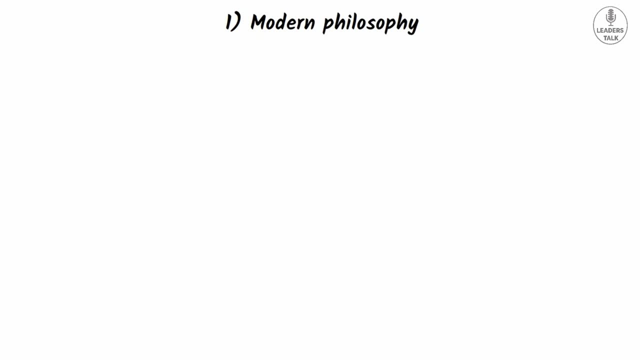 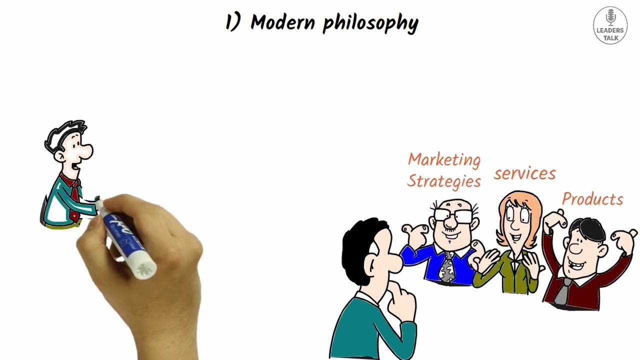 significance. Modern Philosophy. Consumer behavior aligns with modern philosophy, which emphasizes the importance of customer-centric approaches. By understanding consumer behavior, businesses can tailor their products, services and marketing strategies to meet the specific needs and desires of their target audience. This customer-centric approach enhances customer satisfaction and loyalty. 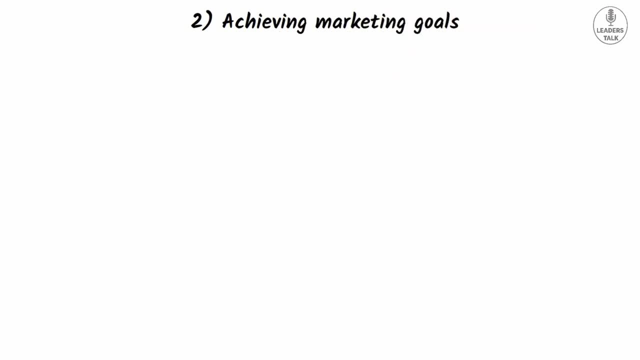 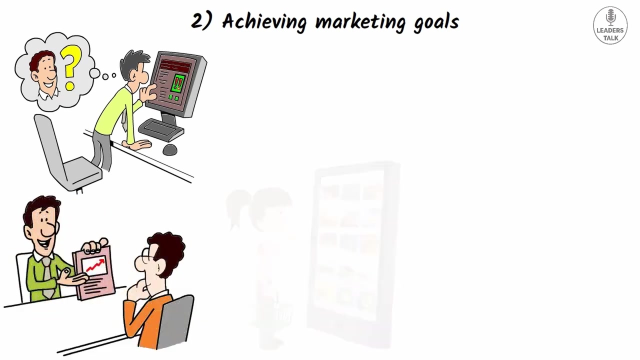 leading to long-term success. Achieving Marketing Goals. Consumer behavior helps businesses achieve their marketing goals. By analyzing consumer preferences and motivations, companies can develop effective marketing campaigns and strategies that resonate with their target market, leading to increased sales and brand loyalty. For instance, understanding consumer behavior. 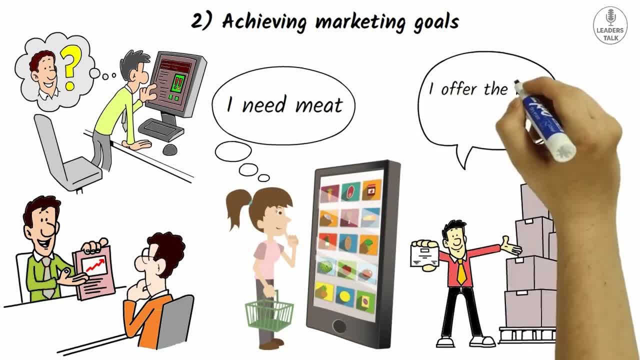 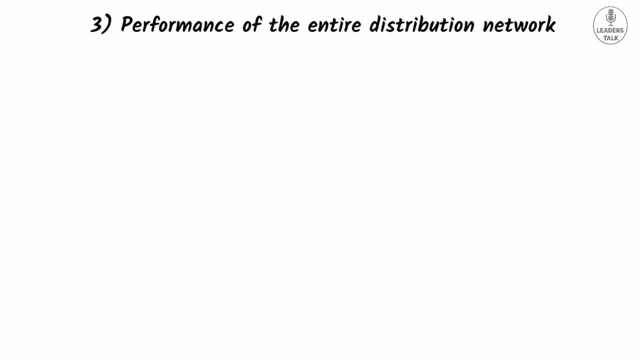 can help a company position its products or services as a solution to consumers' needs or as a way to fulfill their aspirations Performance of the Entire Distribution Network. Consumer behavior also improves the performance of the entire distribution network. When businesses understand their customers' buying habits and preferences, they can provide. 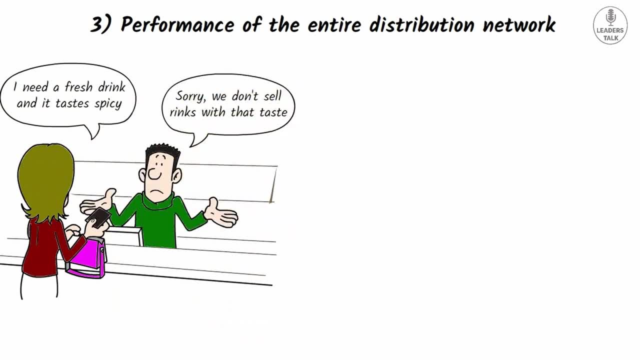 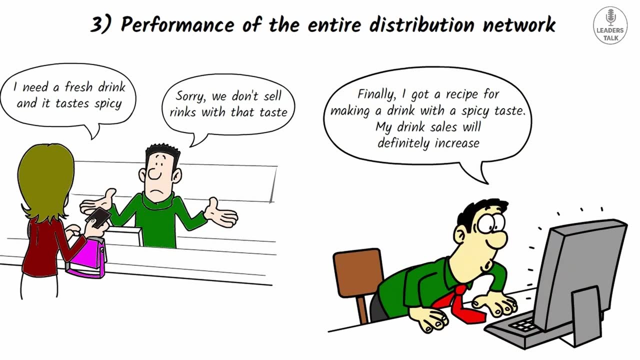 valuable insights to dealers and salespeople, enabling them to enhance their sales and sales performance. Consumer Behavior- Understanding Consumer Behavior. Businesses can enhance their selling techniques and improve customer satisfaction. By aligning their distribution network with consumer behavior patterns, businesses can ensure that their products reach the right customers at the right time. 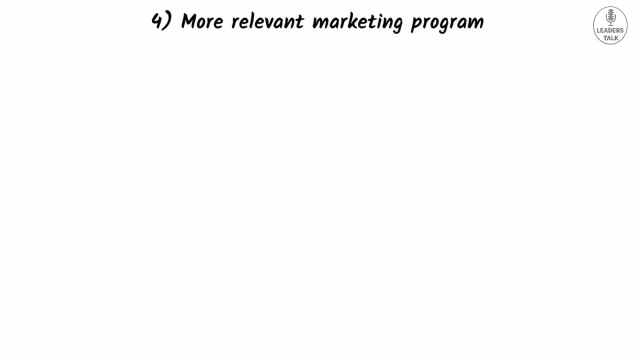 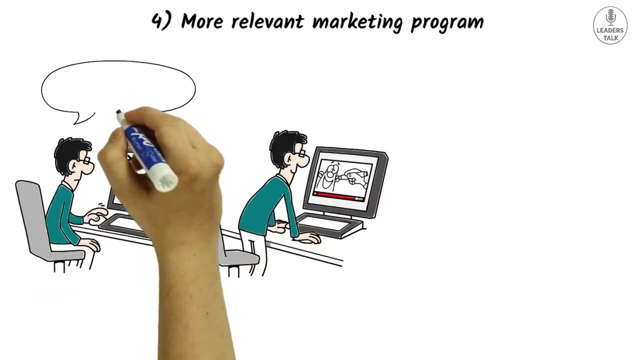 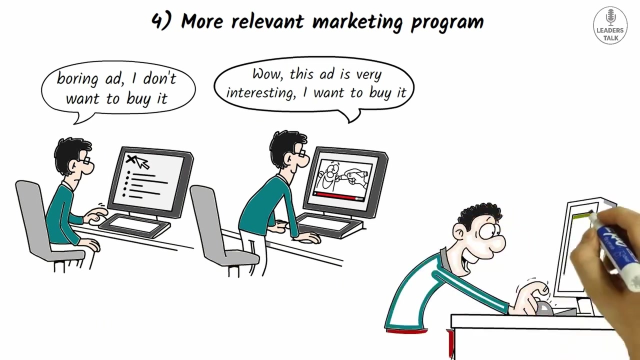 More Relevant Marketing Program. By studying consumer behavior, businesses can develop more relevant marketing programs. This means tailoring their messages, advertising channels and promotional offers to match the preferences, values and lifestyles of their target consumers. By delivering targeted and personalized marketing messages, businesses can create a stronger emotional 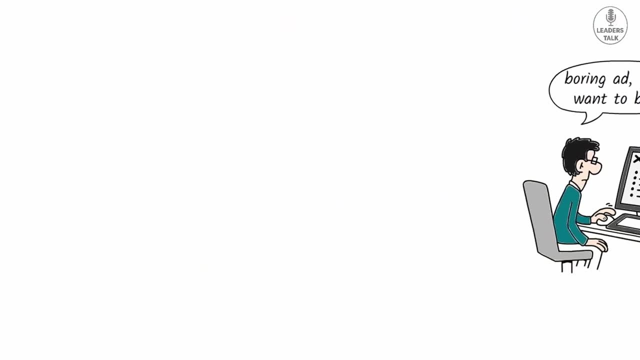 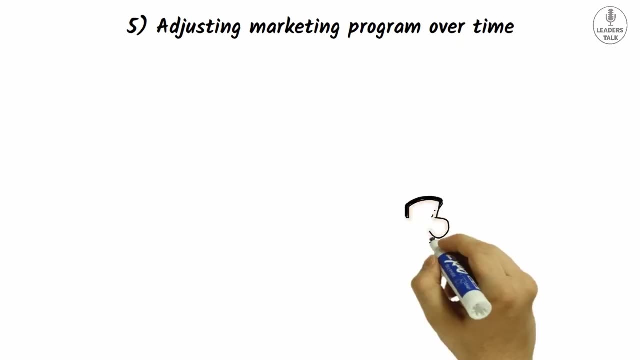 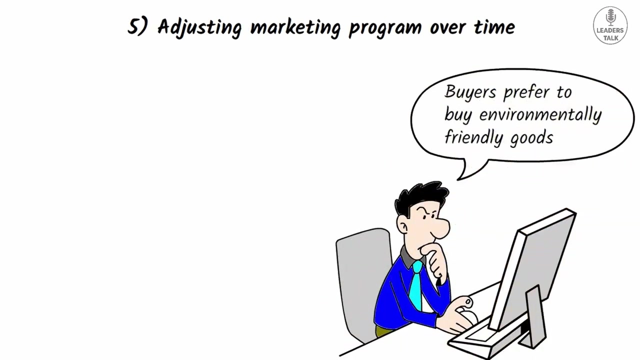 connection with consumers and increase the likelihood of conversion. Adjusting Marketing Program Over Time- Consumer behavior allows businesses to adjust their marketing programs over time. By monitoring changes in consumer preferences and behaviors, companies can adapt their strategies to stay ahead of the competition and maintain their relevance in the market, For example, if consumer preferences shift. 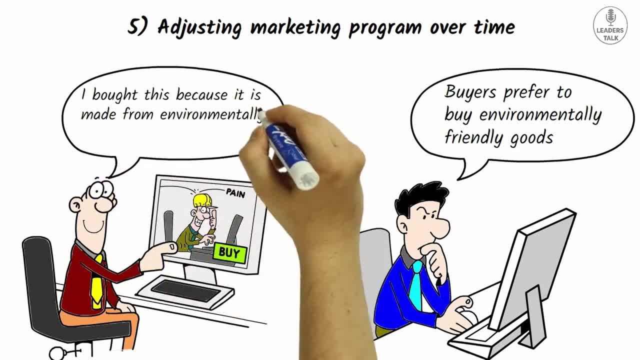 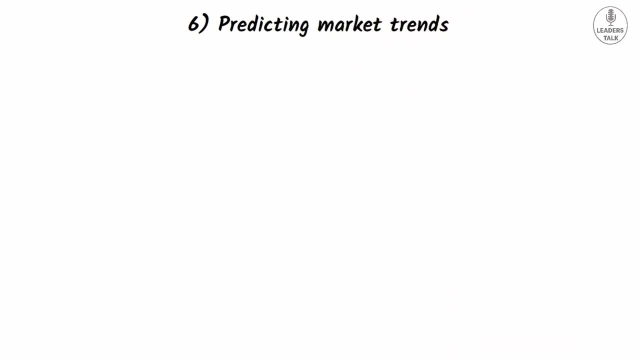 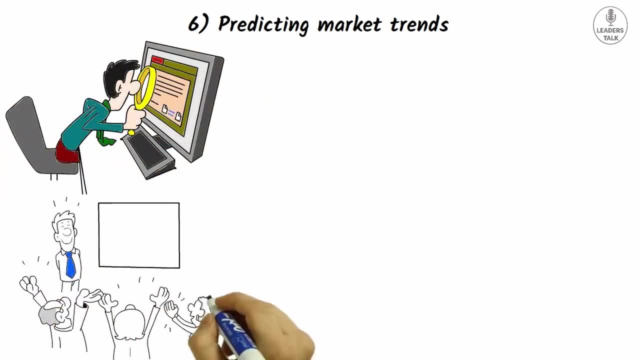 towards eco-friendly products. businesses can modify their marketing strategies to emphasize the environmental benefits of their offerings. Predicting Market Trends: Another benefit of understanding consumer behavior is the ability to predict market trends. By analyzing consumer data and trends, businesses can identify emerging market opportunities and position themselves to capitalize on them. For instance, 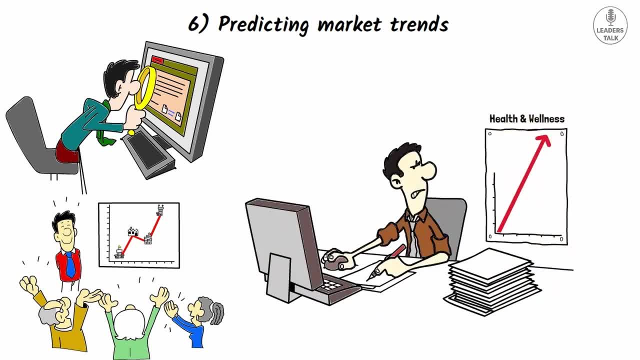 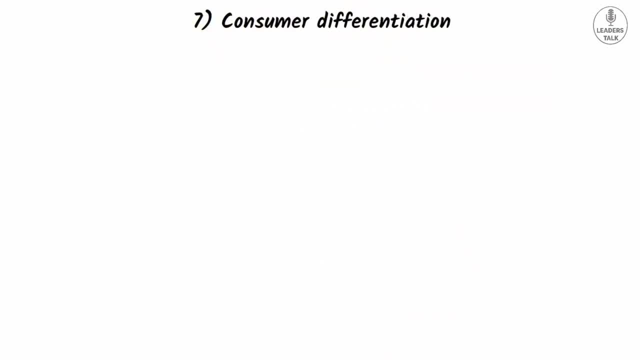 by tracking the growing interest in health and wellness, businesses can develop and market products that cater to this trend, such as organic food, fitness equipment or wellness retreats. Consumer Differentiation: Consumer behavior- helps businesses differentiate their target audience By segmenting consumers based on their preferences. 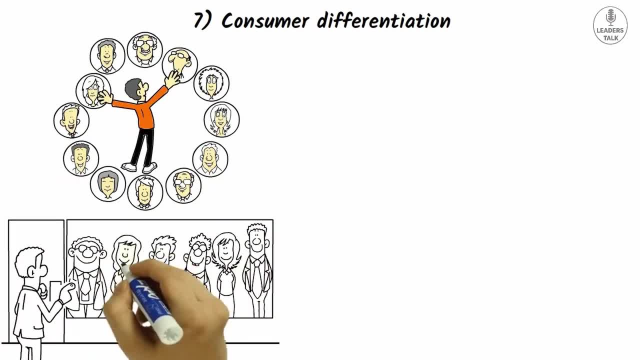 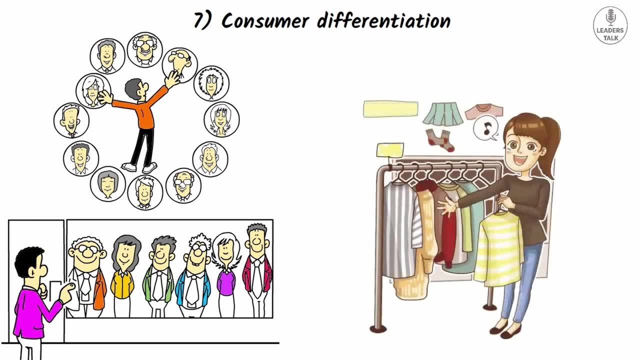 demographics and behavior. companies can develop targeted marketing campaigns that speak directly to specific consumer groups, increasing the effectiveness of their efforts. For example, a clothing retailer may create different marketing strategies for teenagers, young professionals and older adults, recognizing their distinct preferences and buying behaviors. 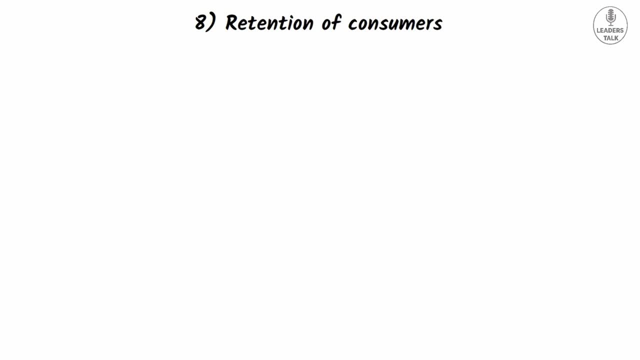 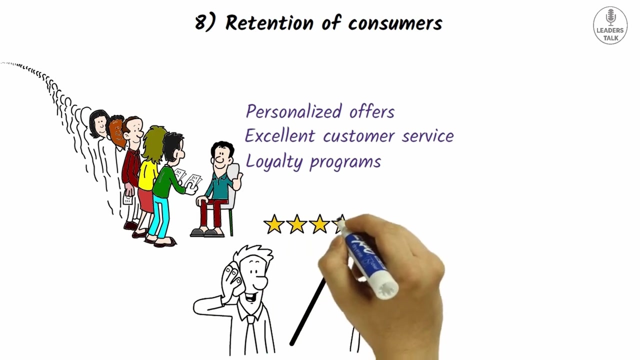 Retention of Consumers. Understanding consumer behavior is crucial for customer retention. By knowing what motivates consumers to remain loyal to a brand, businesses can implement strategies to foster long-term relationships, such as personalized offers, excellent customer service and loyalty programs, By consistently delivering a positive customer experience and addressing their evolving needs. 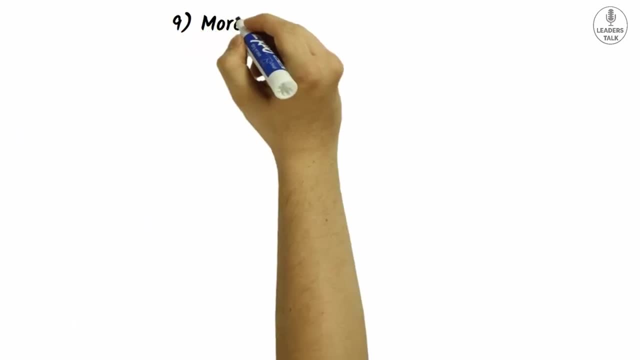 businesses can retain their existing customers and reduce churn More Competitive Advantages. By studying consumer behavior, businesses gain a competitive advantage. They can identify unmet needs in the market, develop innovative products or services to fulfill those needs and position themselves as leaders in their 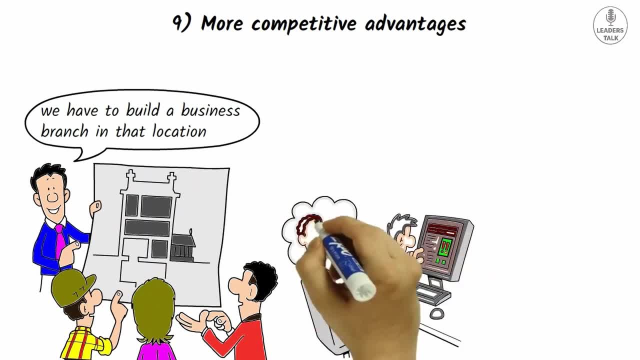 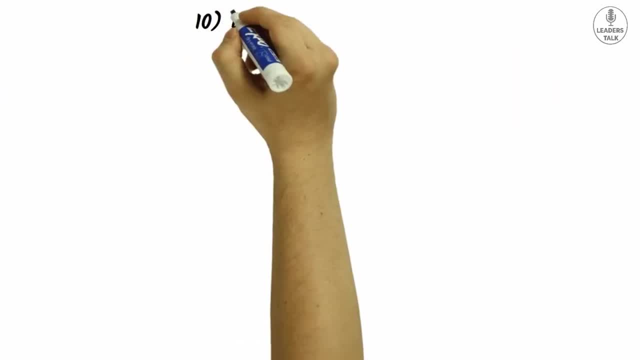 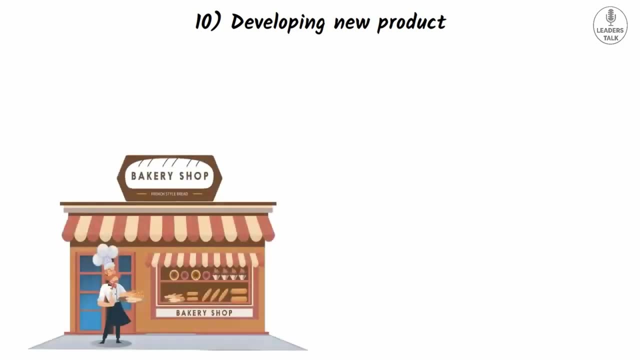 industry. By staying attuned to consumer behavior trends, businesses can outperform competitors by introducing unique features, improving customer experiences or offering superior value, Developing New Products. Consumer behavior research also aids in developing new products. By understanding consumer preferences, businesses can identify gaps in the market and create products that align with the evolving 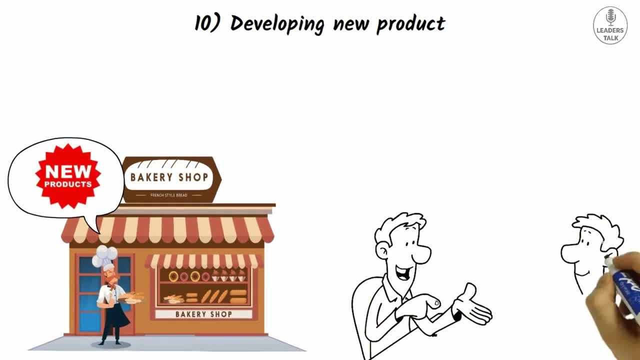 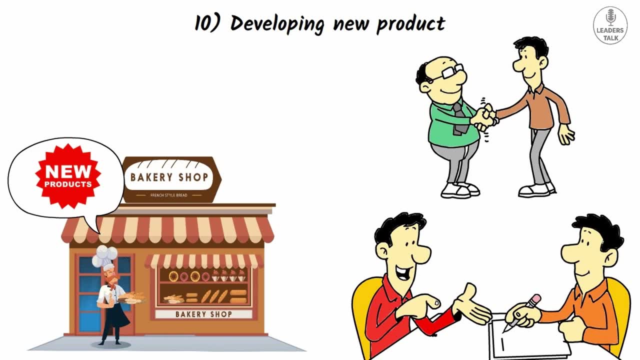 needs and desires of their target audience. By listening to consumer feedback and conducting market research, companies can develop innovative solutions that cater to unmet consumer needs, gaining a competitive edge. Dynamic Nature of the Market: Consumer behavior research recognizes the dynamic nature of the market. 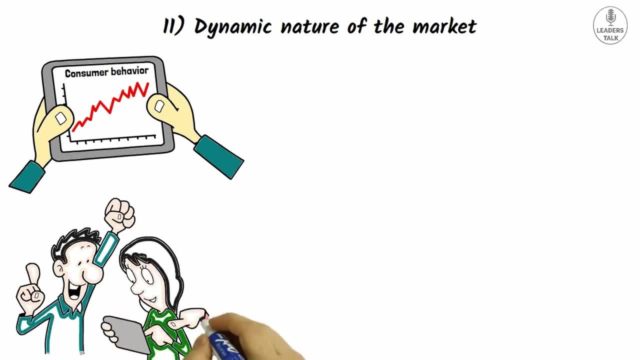 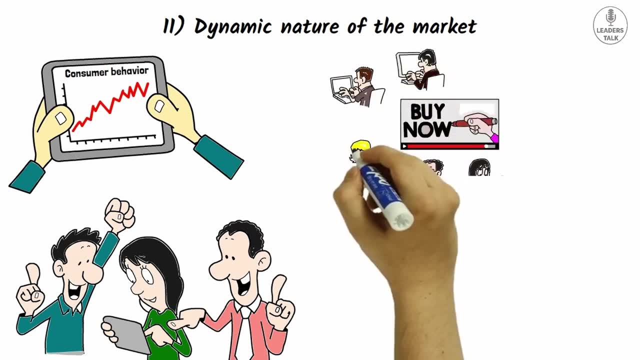 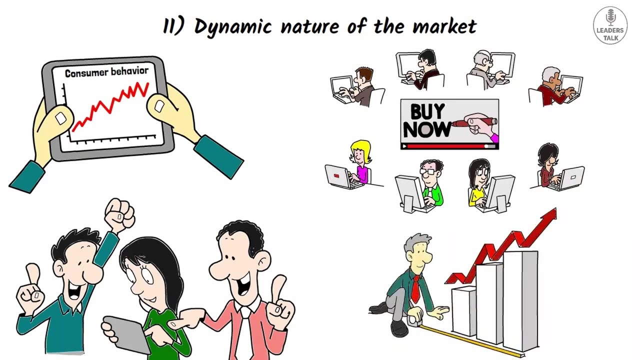 Consumer preferences and behaviors evolve over time, and businesses that stay attuned to these changes can adapt their strategies and remain relevant in an ever-changing marketplace. By continuously monitoring and analyzing consumer behavior, businesses can proactively respond to market shifts and consumer demands, ensuring their long-term sustainability. 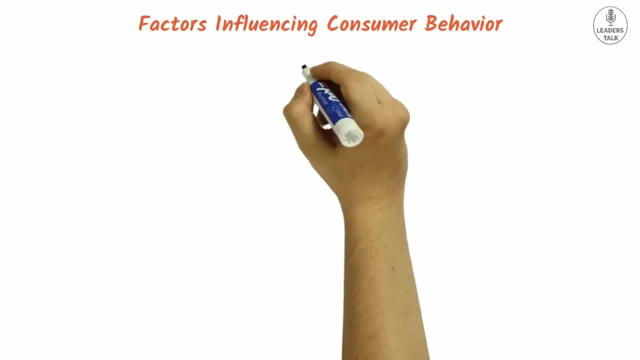 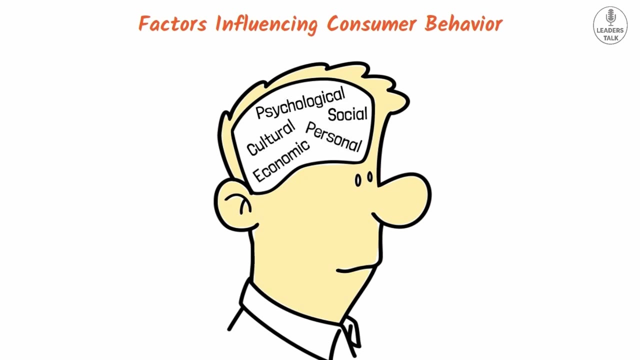 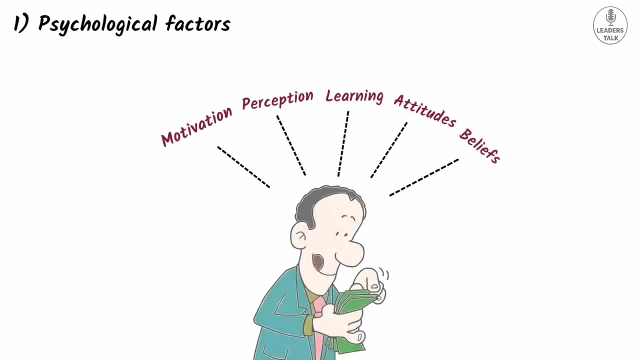 Factors Influencing Consumer Behavior. Now that we've understood the importance of consumer behavior, let's explore the factors that influence it. There are several dimensions that shape consumer behavior. Let's take a closer look. Psychological Factors, Motivation, perception, learning, attitudes and beliefs all influence how consumers 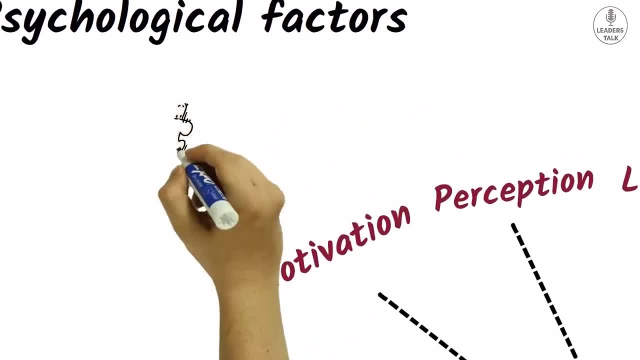 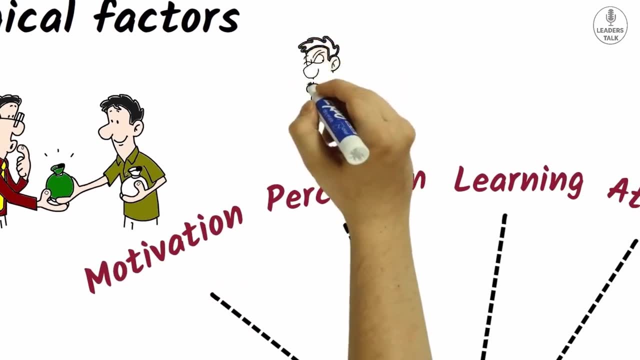 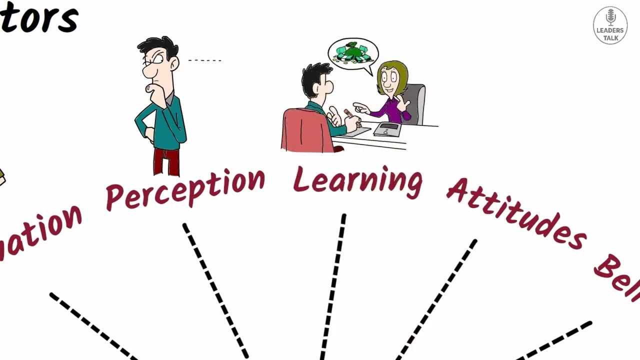 perceive and respond to marketing messages. Motivation is the driving force behind consumer behavior, whether it's the desire for status, pleasure or security. Perception refers to how consumers interpret and make sense of the information they receive. Learning influences consumer behavior through experiences and interactions. 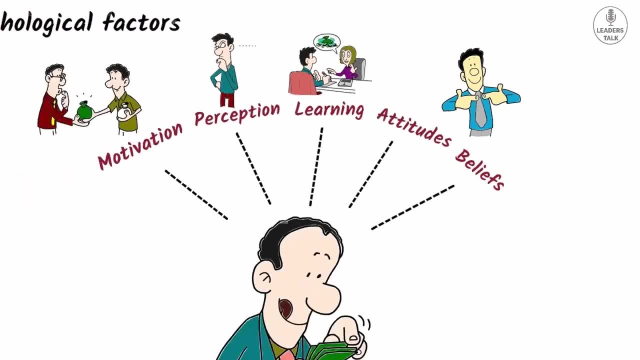 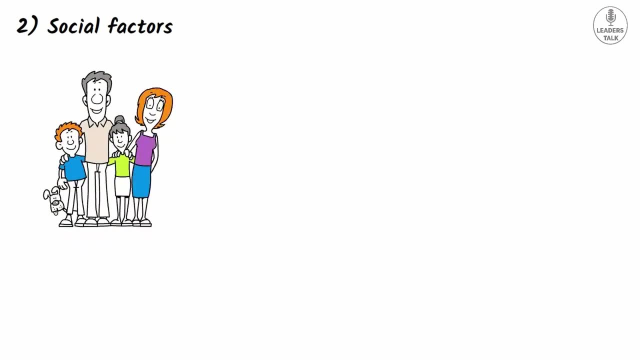 Attitude Interprets consumer behavior through experiences and interactions. Attitude influences consumer behavior through experiences and interactions. Attitudes and beliefs shape consumer preferences and decision-making processes. Social Factors, Family reference groups, roles and status can significantly impact consumer behavior. People are influenced by 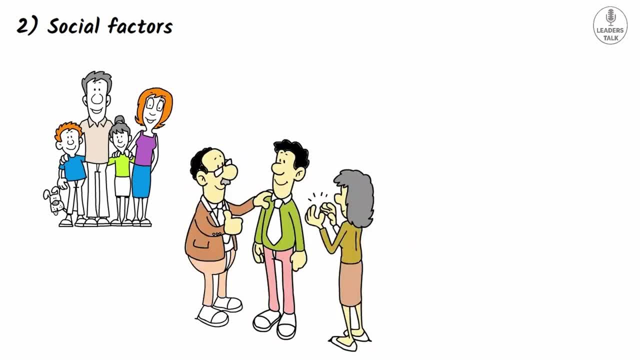 their family members, friends, colleagues and other reference groups in their purchasing decisions. Social roles and status also play a role, as individuals may seek to conform to societal expectations or aspire to a particular social standing. Cultural Factors, Culture, subculture and social class influence consumers' values, beliefs, preferences and 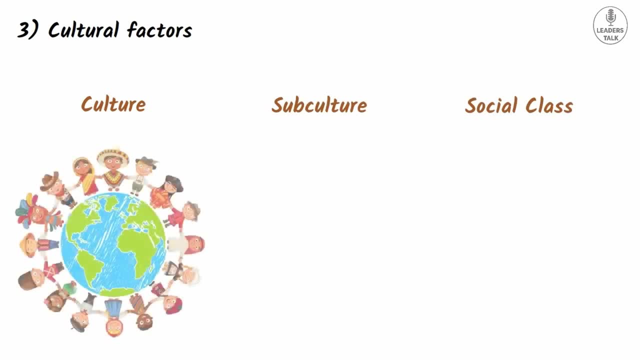 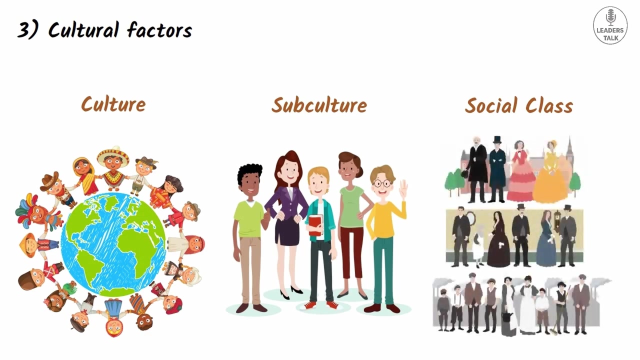 buying habits. Culture encompasses the shared norms, values, customs and beliefs of a particular society, while subculture refers to smaller groups within a culture that share distinct characteristics. Social class, based on factors such as income, education and occupation, also plays a role in shaping consumer behavior. Cultural factors shape consumer preferences. 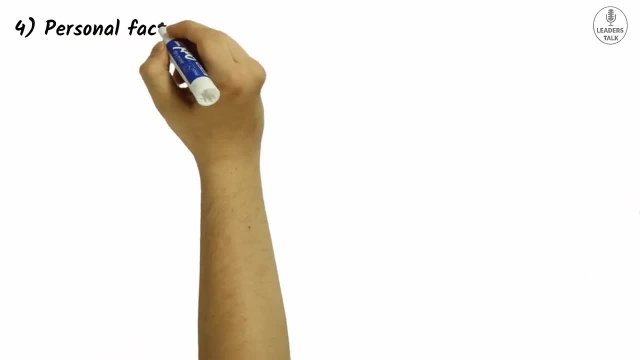 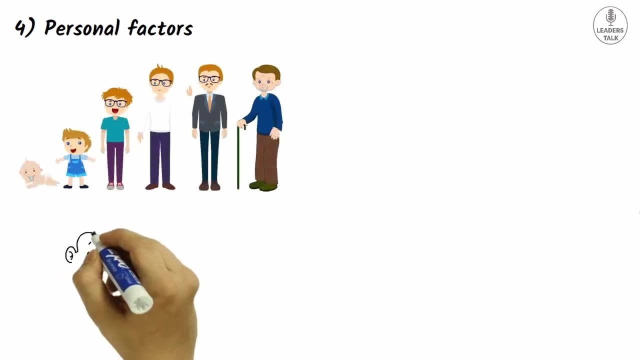 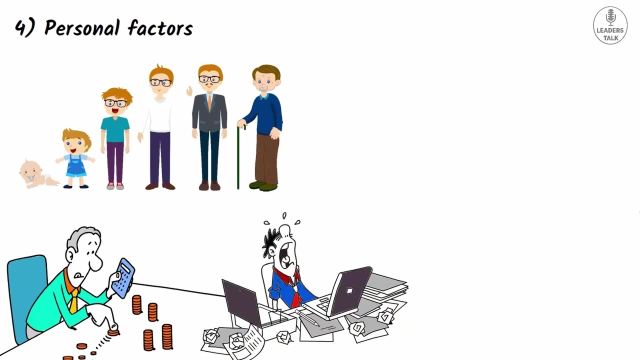 perceptions of value and product choices. Personal Factors- Personal characteristics such as age, income, occupation and lifestyle affect consumer behavior. Different life stages, financial situations and individual lifestyles can significantly impact purchasing decisions and brand preferences. For example, a young 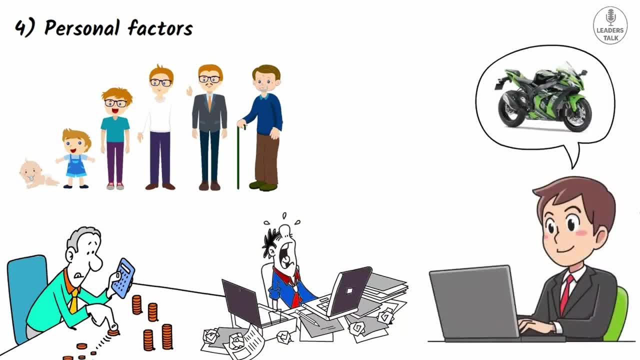 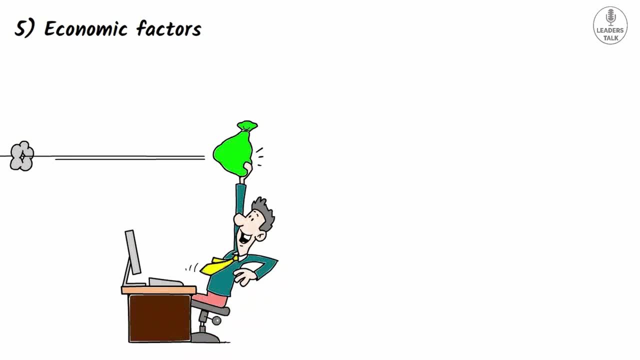 professional may have different preferences and purchasing power compared to a retiree. Economic Factors: Economic factors have a significant influence on consumer behavior. Personal income, family income, consumer credit, liquid assets, savings and income expectations all impact consumers' purchasing power and their willingness to spend. 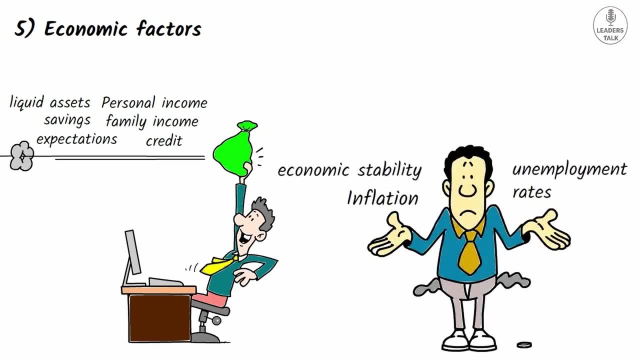 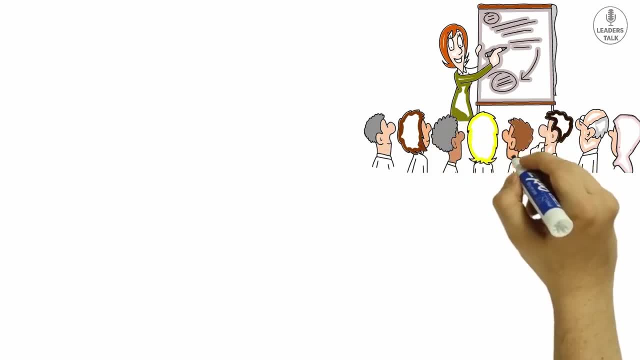 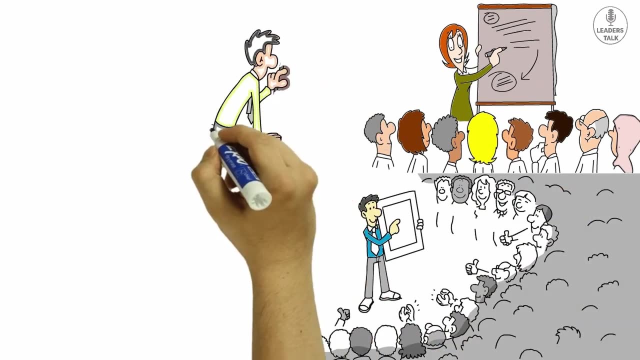 Economic conditions such as inflation, unemployment rates and economic stability can also affect consumer behavior at a broader level. Understanding these factors helps businesses tailor their marketing strategies to specific consumer segments and create targeted campaigns that resonate with their target audience, By analyzing and adapting to the